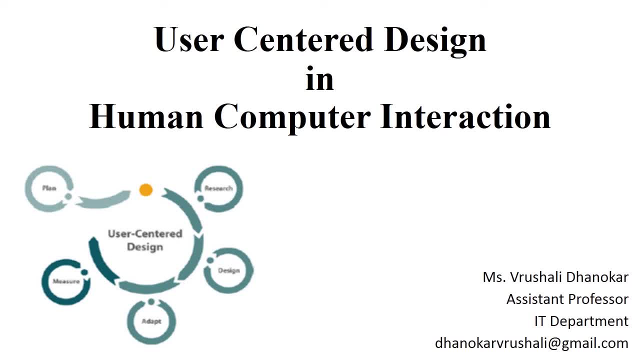 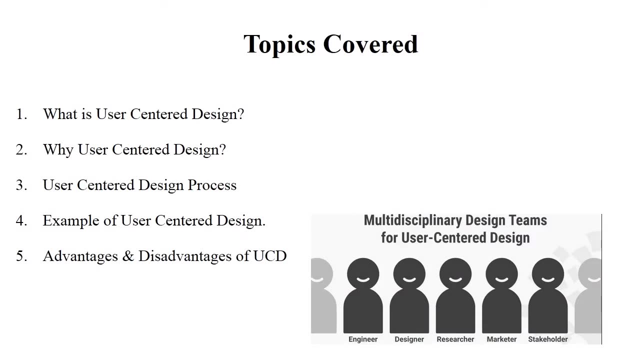 Okay, now in this video, we will learn about user-centered design in human-computer interaction. Okay, so let's see what is meant by user-centered design. Okay, below topics are covered in this video. The topics include: what is user-centered design? why user-centered design? user-centered design process. 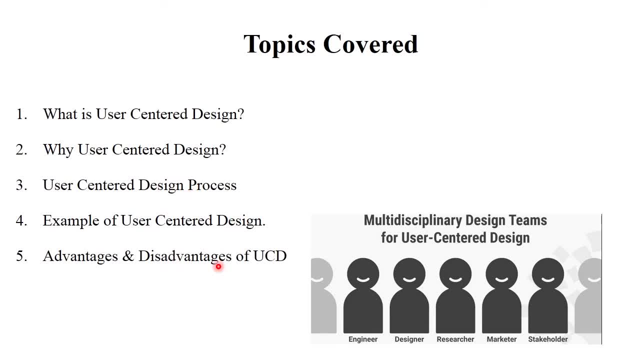 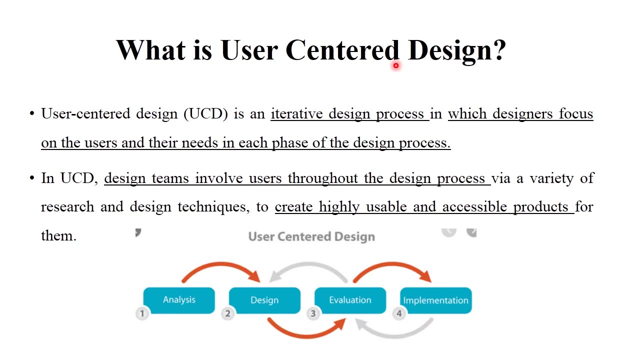 example of user-centered design and advantages and disadvantages of user-centered design. Okay, so let's see one by one: First, what is meant by user-centered design, Okay. next, Okay. so first, what is meant by user-centered design. 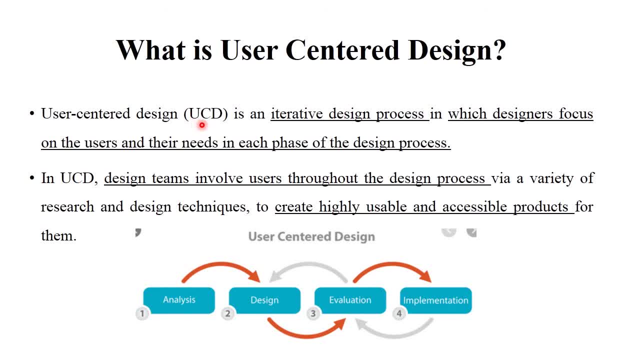 User-centered design is also called as UCD. Okay so user-centered design is interactive design process in which designer focus on the users and their needs in each phase of the design process. Clear. So user-centered design simply means: as per the requirements of the users, as per the need of the customers. 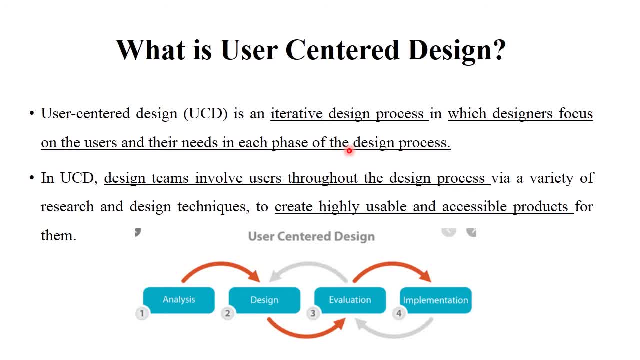 you have to develop your products Clear. So this is the concept of user-centered design. User-centered design team involves users throughout the design process, Why a variety of research and design techniques are available. It also creates highly usable and accessible products for them. 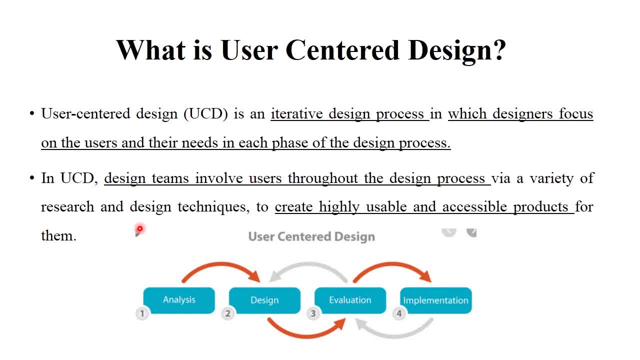 Clear. If we want to involve users throughout the design process. it means that as per the requirements of the user, as per the need of the user, you have to develop your products clear. that's why your products become highly accessible and quality products were developed clear. this is the reason, or this is user-centered design. 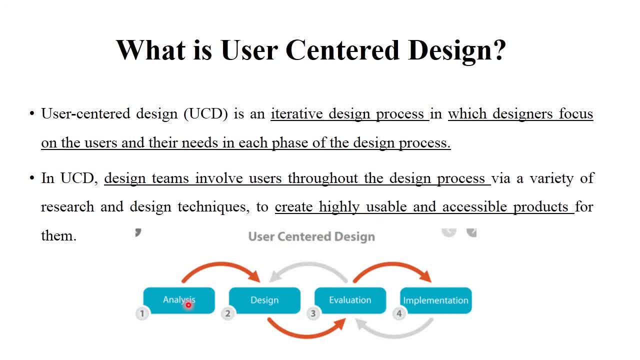 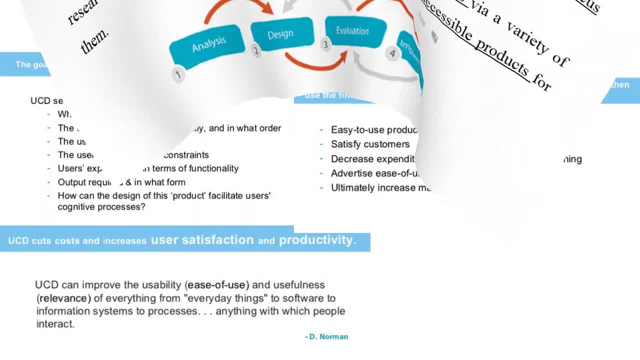 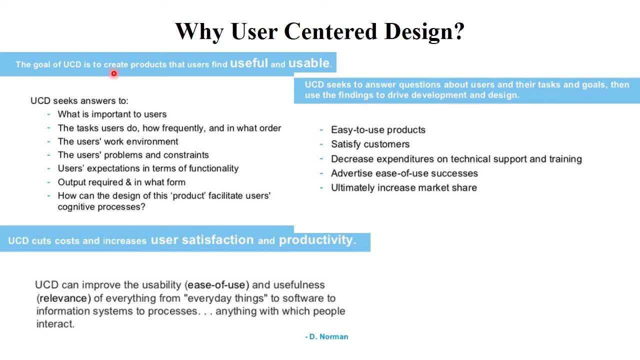 here user-centered design have following process like analysis, design, evaluation and implementation. clear, okay. next, why user-centered design? okay, why user-centered design process is used. so the goal of user-centered design is to create the products. that products are useful and usable. okay, i already told you, user-centered design means each and every generation or each and every people, whether it is. 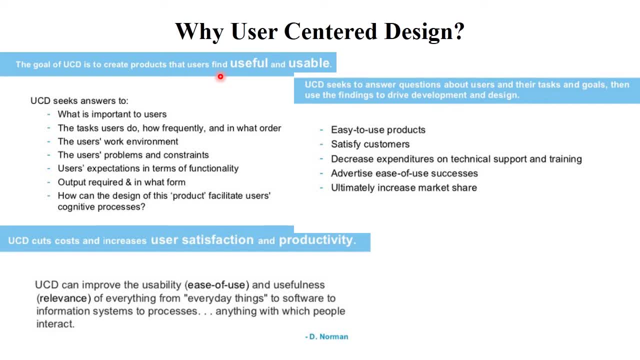 technical people and non-technical people. each and everyone use the products as per their requirement. okay, that's why user-centered design process is used. user-centered design: it seeks answers to what is importance of users, the tasks users do, how frequently and what order the user's work. 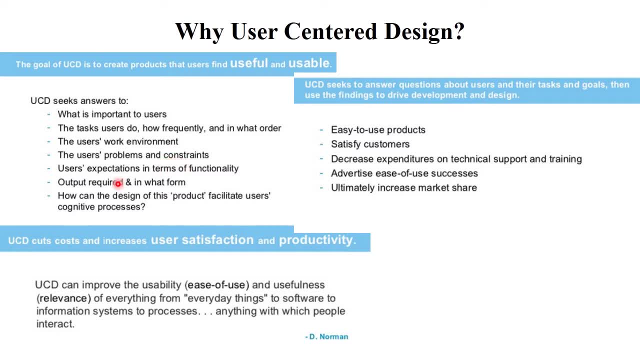 environment. the user's problem and constraints. users expectation in terms of functionality, output required and in what form. how can the design of this product facilitate users and cognitive processes? okay, so this user-centered design given answers to these six questions, to all those questions. clear user-centered design seeks to answer the question about. 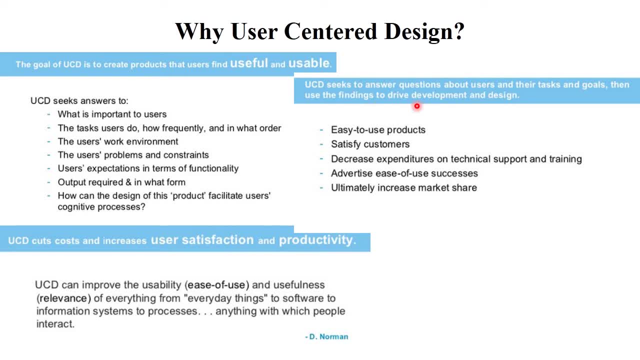 users and their tasks and goals. then use the finding to drive development and design. okay, through user-centered design, finding the drive development and design. okay. so through user-centered design, easy to use the product, it satisfy the customers, decrease expenditure on technical support and training. it also advertise ease of use successes and ultimately increase market share. 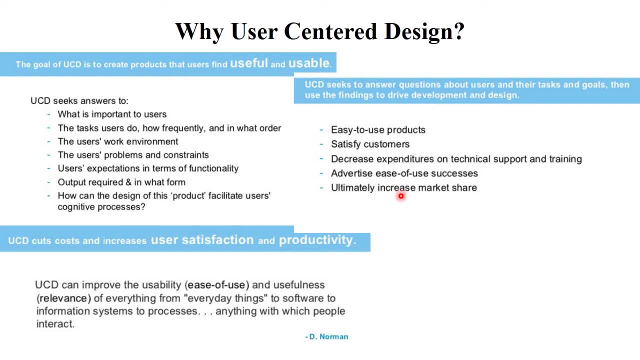 okay, because each and every process or each and every phase, users are involved. that's why this benefits are gained via user-centered design. okay again, user-centered design cuts cost and increase user satisfaction and productivity. if you you have developed a particular product as per the user's need or requirement, then you 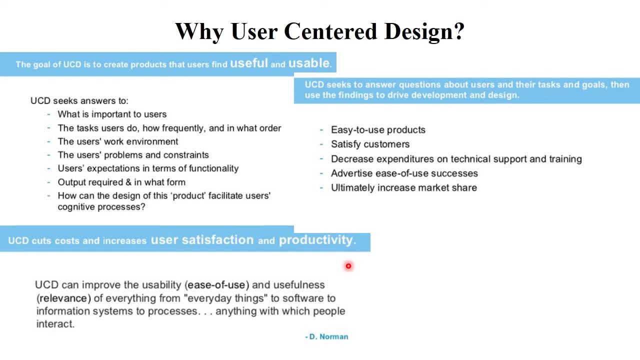 you users are satisfaction generated, okay, and your productivity increased. clear, user-centered design improve the usability. that is ease of use and is usefulness. that is relevance of everything from everyday things, the software to information system to process anything with which people interact. clear. so this is the advantages of user-centered design: clear, okay. next, 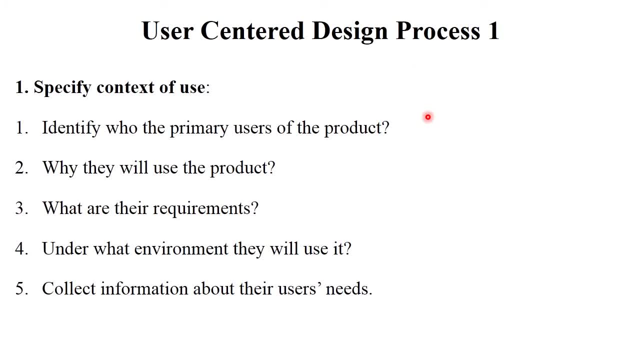 so users? user-centered design process. how user-centered design process is generated. the first step is specify context of use. okay, in this step, you need to identify who the primary users of the product. okay, so just consider that you work as a developer or you work as a designer. clear, then. first thing, 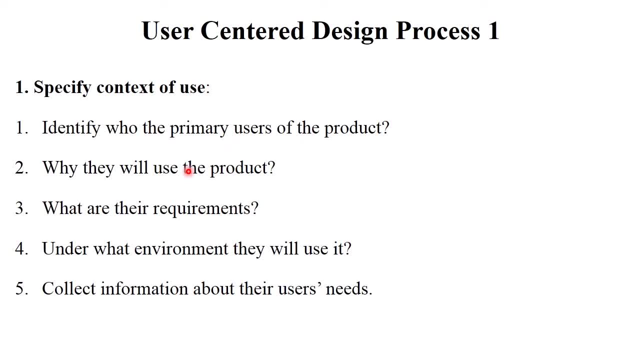 is to identify who the primary users of the product and why they will use the product. you must know that users, age, their requirements, their need, their education or each and everything about your customers and users clear and why they will use the product. is this product used for educational purpose? for financial purpose, for hospital or bank related purpose? you have to clear about that. clear, then: what are their requirements? you have to focus on requirements and need of the customers or users. clear, then, under the 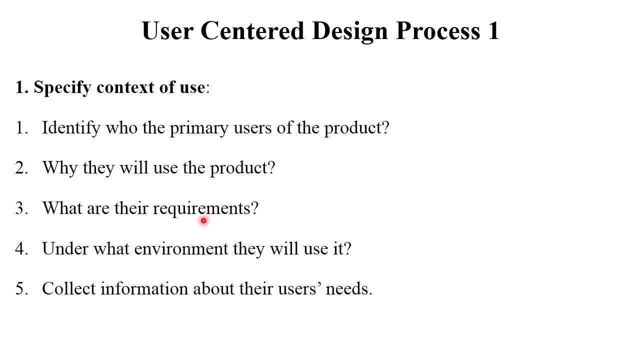 what environment they will use it: okay. collect information about their users need: okay. collect information about the users need: okay. so this is the first step: to identify users, to identify requirements and needs of the customers. here this is a four stay okay. next, the second type of user centered design process is specify requirements. 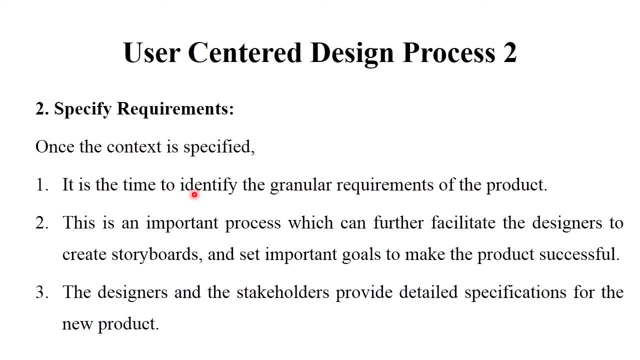 user-centered design process is specifically required. user-centered design process to further defining user Island. so 엄청 descriptive. the personal experience of the consumer is especially important because we know that customers operate environment most likely will not be particles or influences. So please remember this: In the first step, you just identify your customers and specification of your customers. 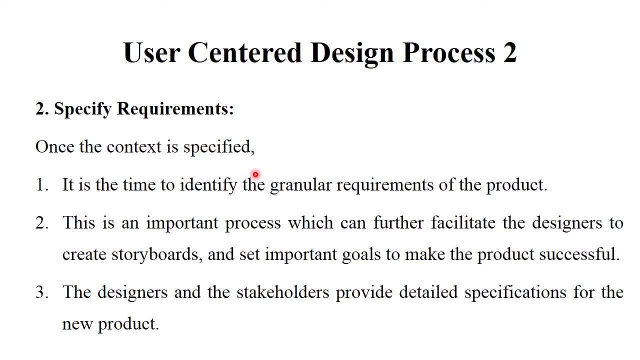 Now second step is system requirement. Once the context is specified, it is the time to identify granular requirements of the product. You have to know each and every requirements related to the product, For example, WhatsApp. So what are the requirements for WhatsApp? 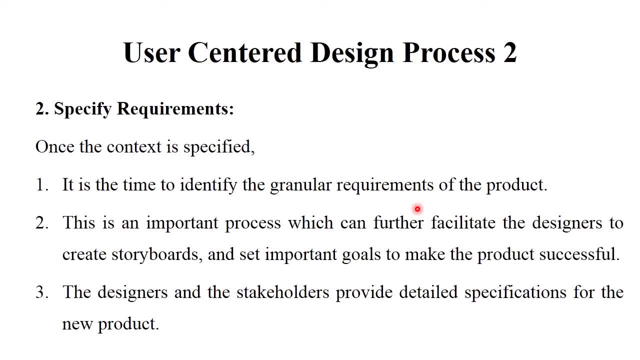 That is chatting functionality, audio video, then post status again- payment. These type of functionalities are included in WhatsApp, So you have to know requirements of the product. This is an important process which can further facilitate a designer to create storyboard and set important goals to make the product successful. 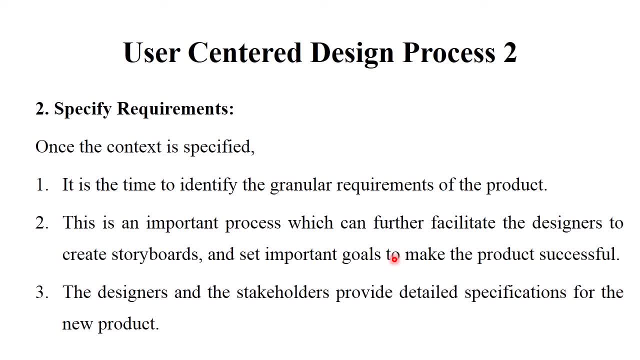 These all types of requirements can be provided to the designers for design the quality product, The designer and stakeholder provide detailed specification for the new product Clear. So first step is to identify customers and second step is to identify requirements of the product. 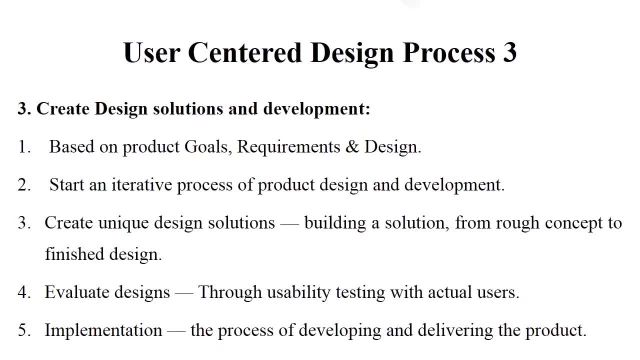 Clear, Okay. next. The next step is create design solution and development. Okay, You know about your customers, You identify the requirements. Then third step is create design solutions. Okay, Based on product goals, based on product requirements, you have to design your product. 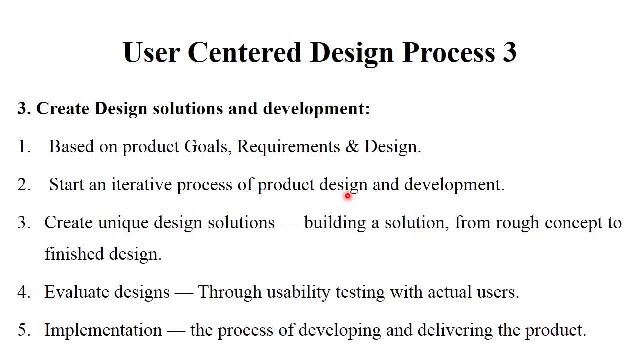 Clear. Start an iterative process of product design and development. Create unique design solutions, building a solution from rough concept to finish the design. Okay, First you have to design your product in rough way, Or one of the most simplest way is paper and pencil used. 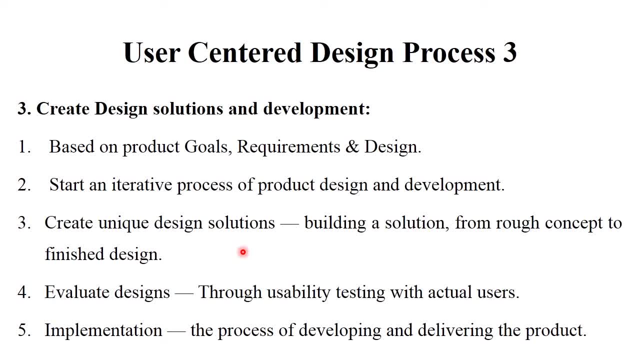 Okay, So you have to create unique design solution. You have also. You have to use activity diagram, XML diagram, use case diagram, then a state transition diagram. This type of design techniques are used to design the product Clear, To evaluate a designs through usability testing with actual users. 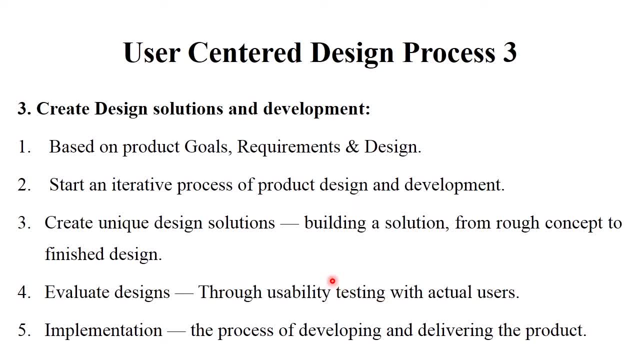 Okay, And after design, this design is provided to the developers in development team Clear. So implementation is one of the process of developing and delivering the product. Okay, For implementation purpose, You have to know which type of hardware, which type of database or which type of framework language is used. 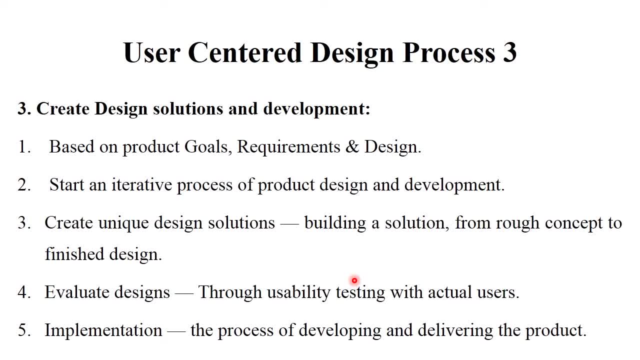 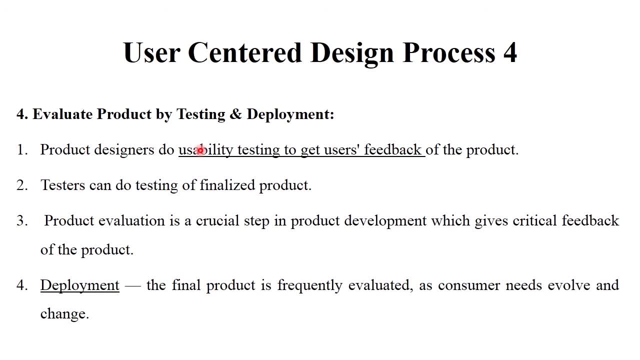 Okay. So for that purpose, you have to develop your product according the design Clear. Okay. Next Last step is evaluate product by testing and deployment. Okay, After developing your product, you have to test your product. Okay, In each and every phase, users are involved. 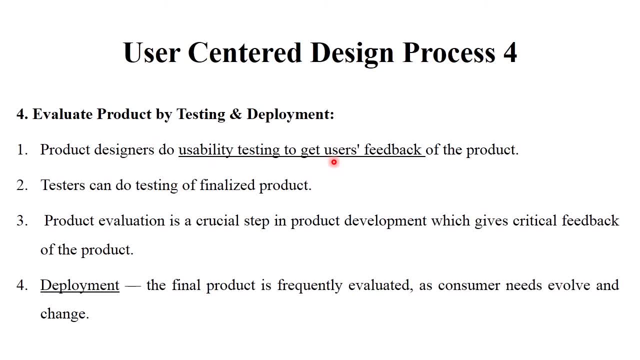 Okay, So product designers, Testers, do usability testing to get user's feedback of the product. Okay, And testers can do testing of finalized product. Mainly, there are three types of testing: unit testing, integration testing and usability testing. 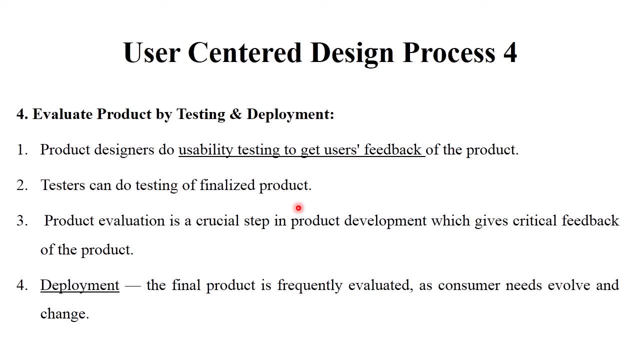 Okay, This is general approach. Okay, In unit testing, each and every modules are tested- Okay. Integration testing: overall products will be tested- Okay. And usability testing to get the user's feedback of the product: Okay. This type of testing will be done on finalized product. 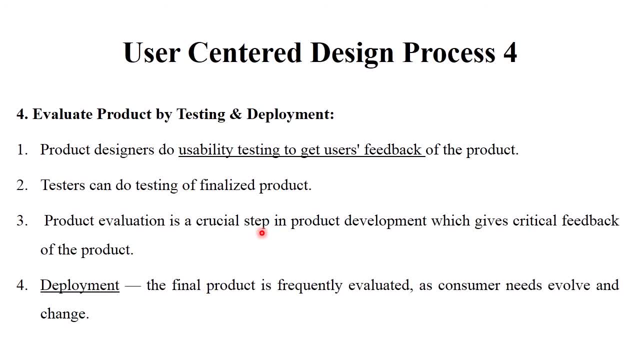 Okay, Then product evaluation is one of the crucial step in product development, which gives critical feedback of the product Clear After the testing deployment part is done. Okay. Deployment means the final product is frequently evaluated as consumer needs evolve and change. 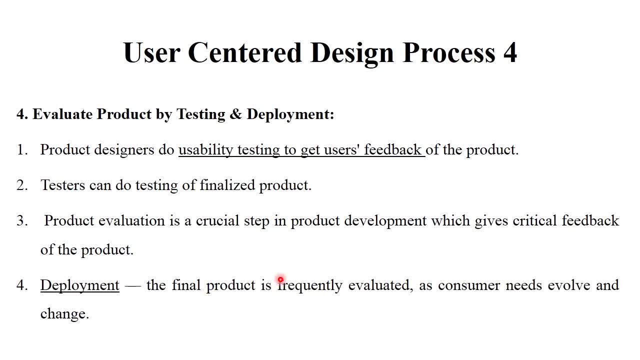 Okay. So requirement phase, planning phase, design, then implementation, testing and evaluation. Okay, Testing and deployment. Each and every phase, users are involved, Clear. So this is a user-centered design process. This process is just like software development: lifecycle phase. 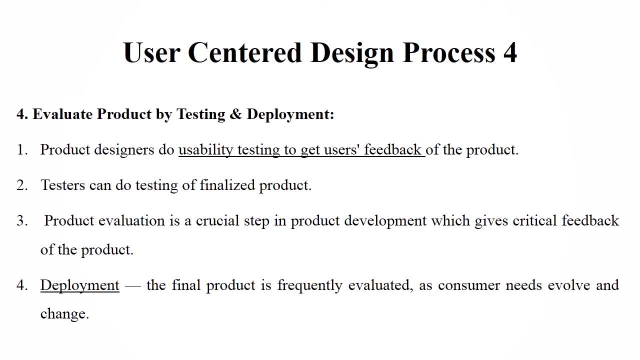 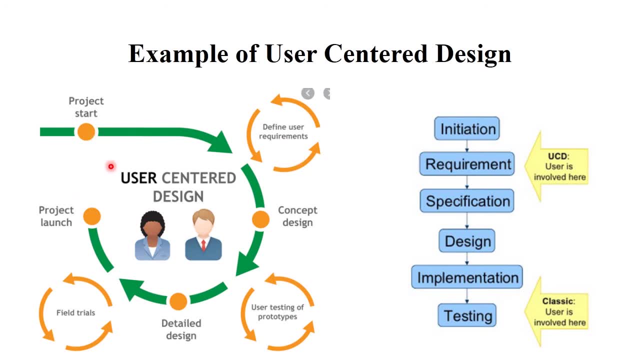 Clear. Okay Next. See here. This is the example of user-centered design process. See here Just one example: Projects start here. Okay. Then define user requirements. After the requirements gathering: concept of design: Okay. After that, user testing of prototypes. 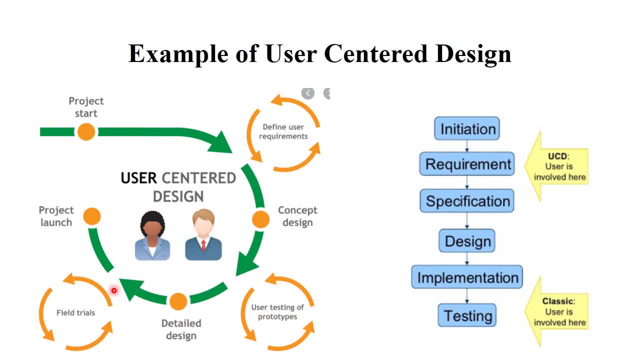 Okay, Then detailed design. After that there is implementation or field of trials, or testing- Clear, And at last, project launch: Okay, And in this complete phase, users are here, which is called as user-centered design- Clear. 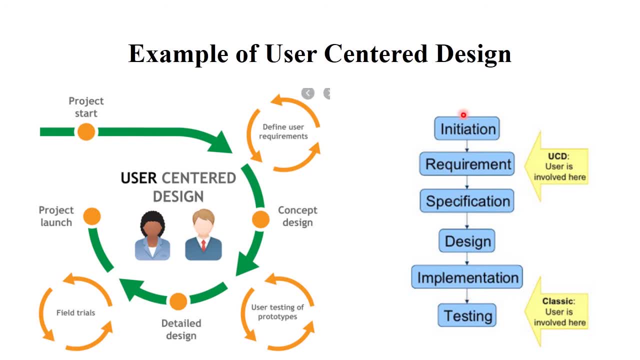 Okay, See here These are the sequence of phases, That is, initiation, Requirement, Specification, Design, Implementation And testing. Okay, So initiation, Requirement And specification, These three phases- users is involved, Clear And after that, testing phase: users are involved. 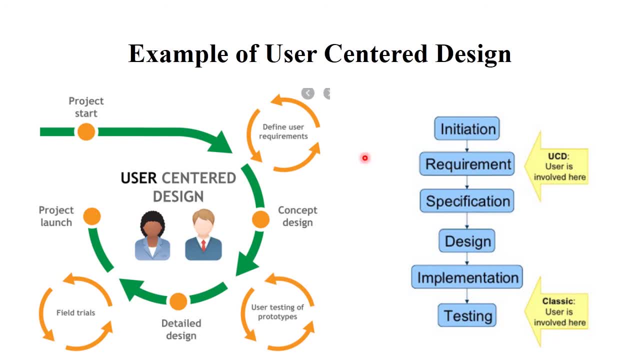 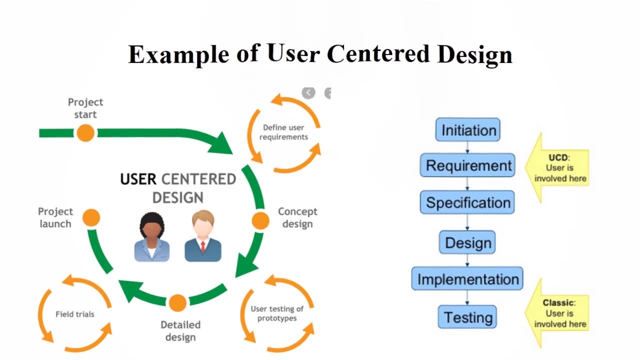 Clear, So this is the approach of user-centered design process. Okay, So by using UCD approach, you have to develop your product more usable and more quality. Qualitable product. Clear, Okay. Next, Advantages and disadvantages of user-centered design. 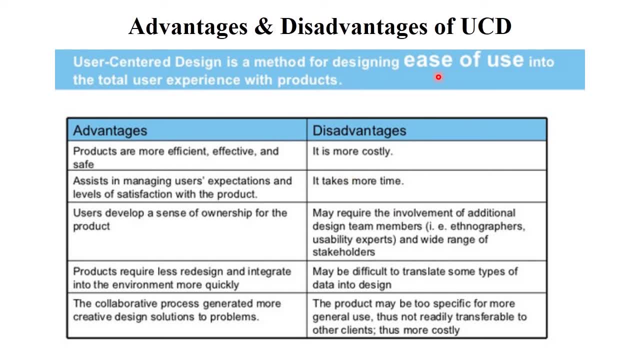 User-centered design is a method for designing the ease of use into the total user experience with product. So the advantages of user-centered design is: products are more efficient, effective and sane. Okay, Assist in managing the user's expectation and levels of satisfaction with the product. 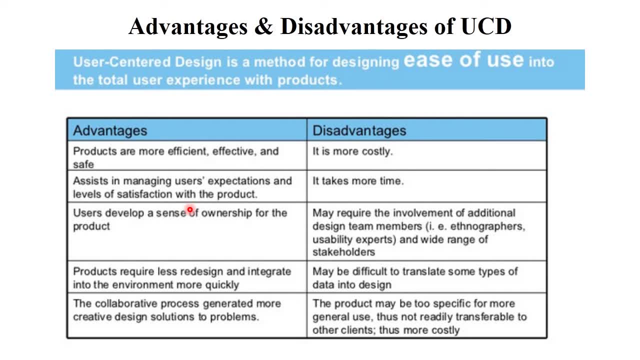 This is one of the main advantage of user-centered design: That users get satisfied. Okay, Users develop a sense of ownership for the product. Products require less redesign and integrate into the environment more quickly. Right, The collaborative process generated more creative design solutions to problem.